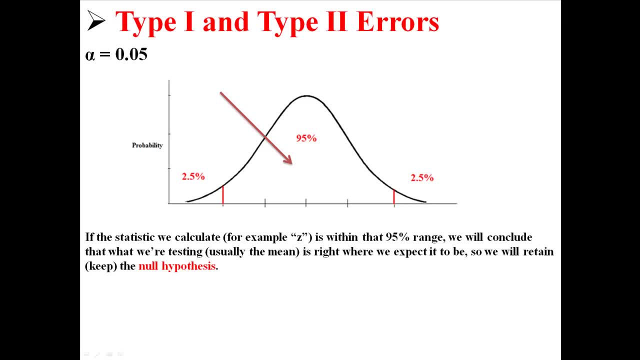 And so we will retain or keep the null hypothesis. The mean is right, where we assumed it would be, so we're going to stick with our initial assumption. Now, if the statistic we calculate is outside of that 95% range, 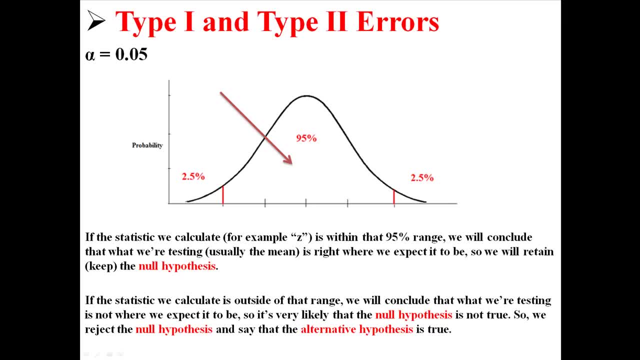 we will conclude that what we're testing is not where we expect it to be, And so it's very likely that the null hypothesis is not true. So we're going to reject the null hypothesis and say that the alternative hypothesis is true. Basically, we're going to say: okay, the mean is in this area. 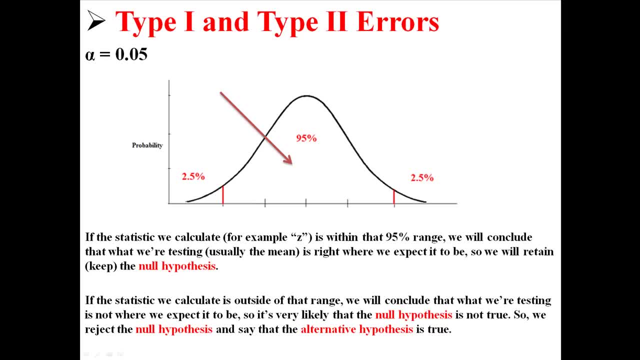 and it's so unlikely for the mean to show up here that it's probably here because it is different from the null hypothesis. It's different from what we assumed it would be, So we can conclude that the alternative hypothesis is probably true. It's probably different. 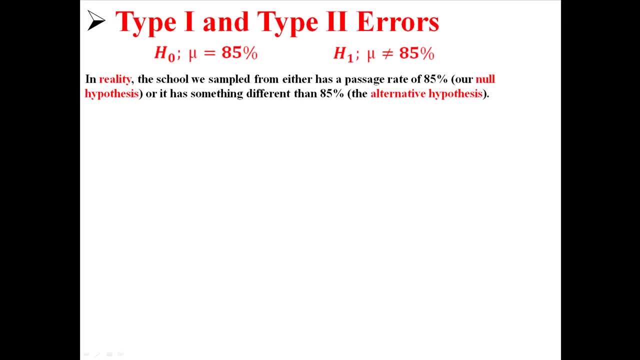 So we have the hypothesis. So we have the hypothesis here And now. in reality, the school we sampled from either has a passage rate of 85%, which is our null hypothesis, or it has something different than 85%, which is our alternative hypothesis. 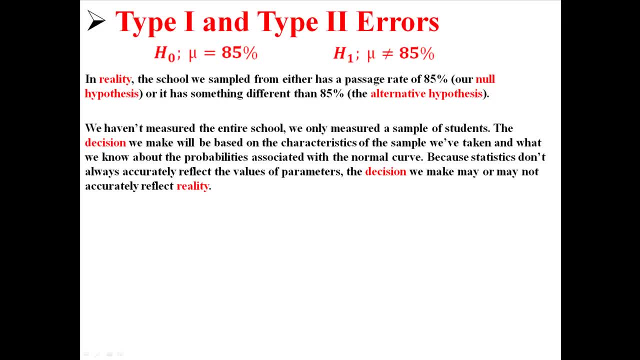 So we haven't measured the entire school, We only measured a sample of students. The decision that we make will be based on the characteristics of the sample we've taken and what we know about the probabilities associated with the normal curve, Because statistics don't always accurately reflect the values of parameters. 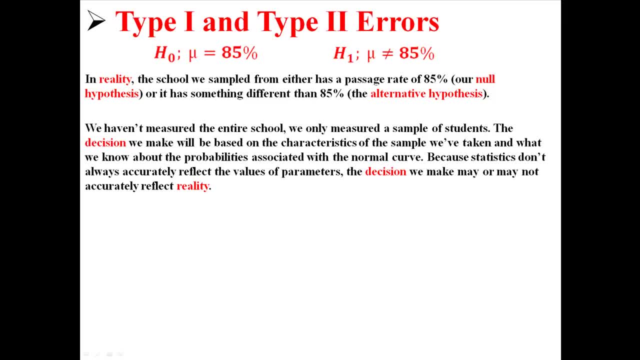 the decision we make may or may not accurately reflect what's real. It may not accurately reflect reality. So, in reality, the null hypothesis is either true or false And we're going to make a decision about whether that null hypothesis is true or false. 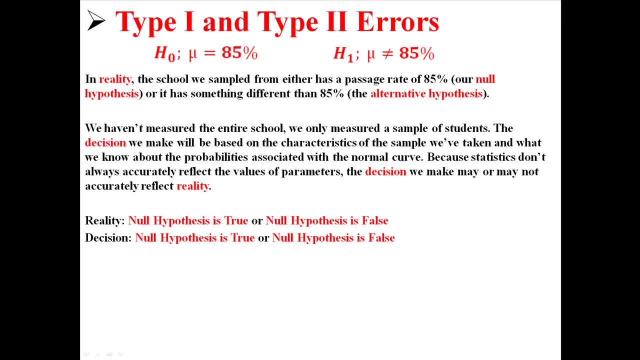 So we could be right, we could be wrong. There are four possible things that could happen. Outcome one is that we reject the null hypothesis when in reality it is false. So what's that saying? What it's saying is that we reject the null hypothesis when we're supposed to. 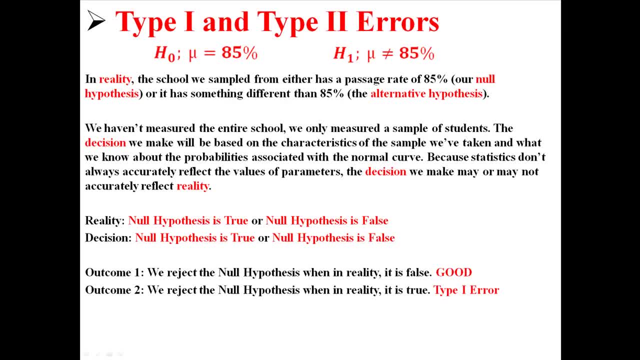 That's good Outcome. number two is that we reject the null hypothesis when in reality it is true. So what we're saying is we're saying the null hypothesis is false when actually in real life, it was true. 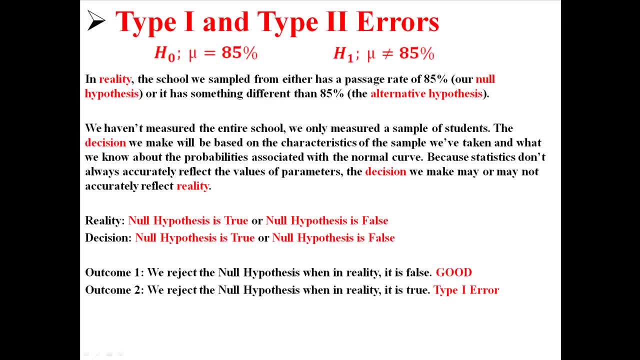 That means we made a mistake, and that mistake is called a Type I error. The third outcome is that we retain the null hypothesis when in reality it is false. So we're saying, okay, we found it to be true.